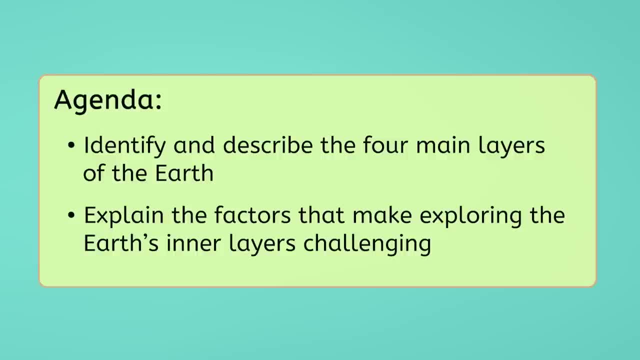 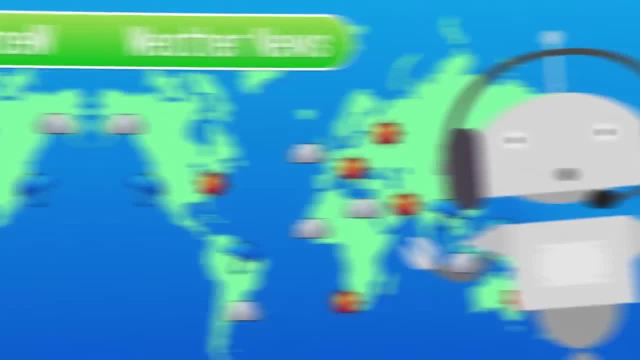 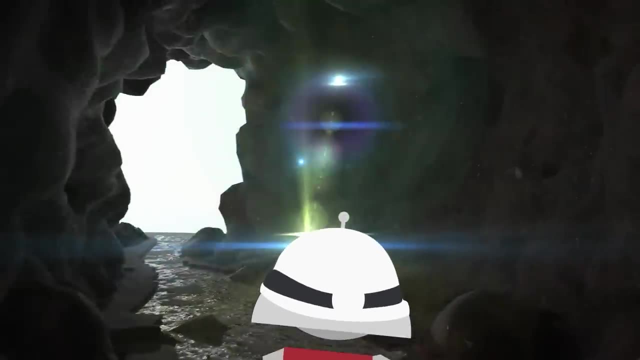 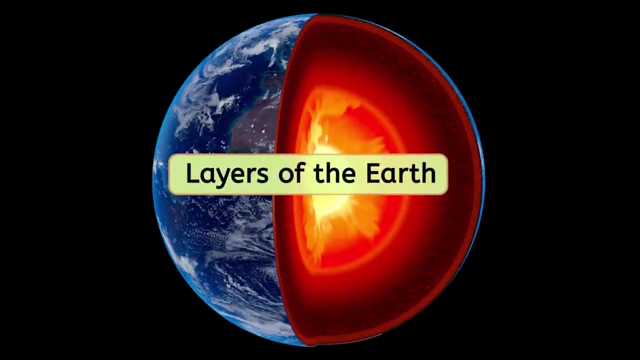 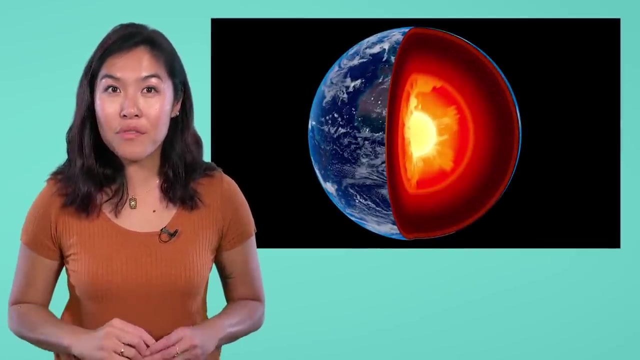 and explain the factors that make exploring the Earth's inner layers such a challenge. Let's get started. The Kola Superdeep Borehole only made it into the first layer of the Earth, called the crust. This is the layer we call home. 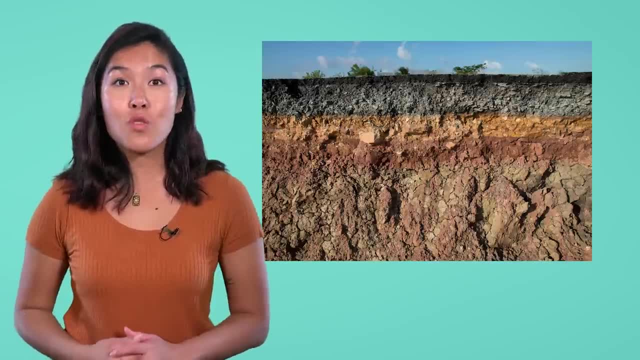 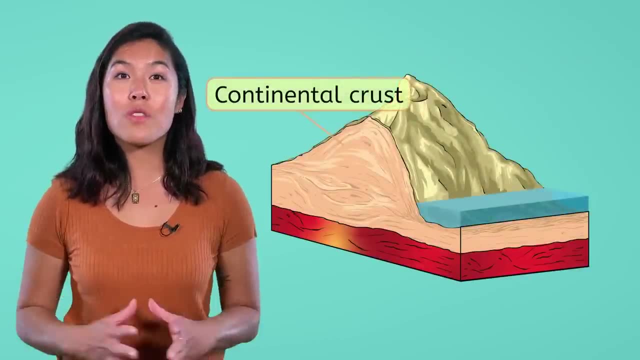 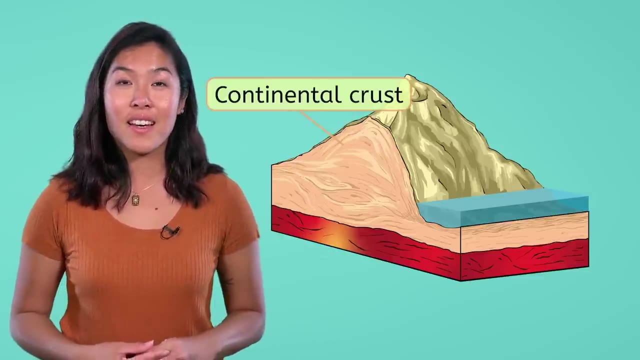 The crust is made of a mixture of different kinds of solid rocks and minerals. It's also the thinnest of Earth's layers by far. The continental crust, or the parts of the crust beneath land masses, varies from about 25 to 50 miles thick, But the oceanic crust under the oceans is as thin as 3 miles. Our planet's crust isn't just the layer we live on, it's also the only layer we've actually explored at all. The Kola Superdeep Borehole made it less than halfway through this layer. If it had kept digging deeper, the next layer it hit would have been the mantle. 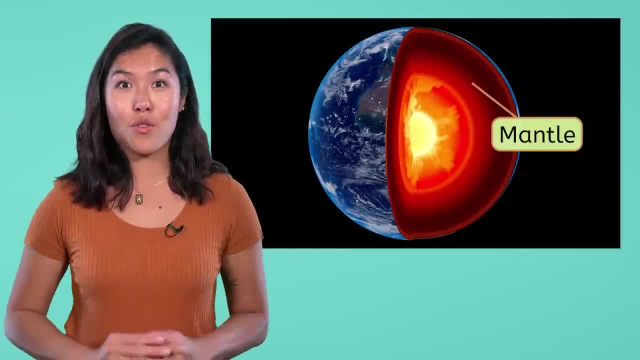 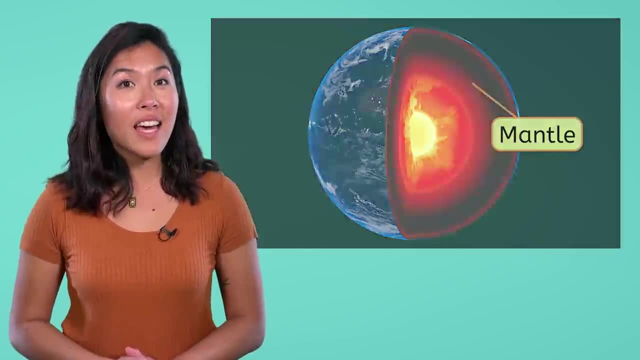 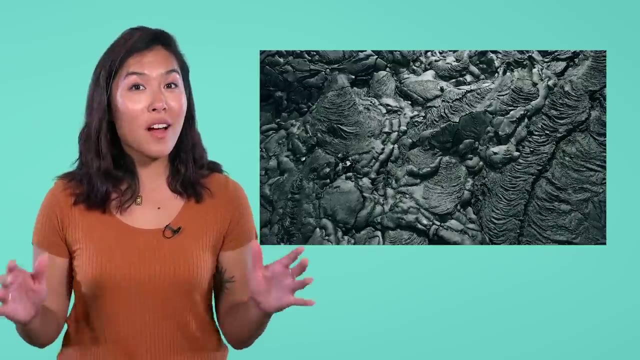 The mantle is the layer that lies beneath Earth's crust At a whopping one thousand eight hundred miles thick. it's by far the thickest of our planet's layers. The mantle is made of rocks that are denser and heavier than the rocks in the crust. 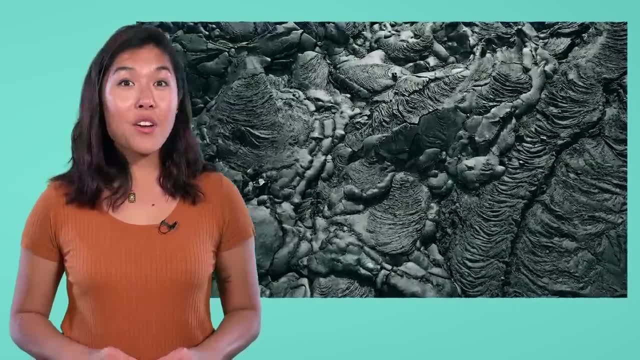 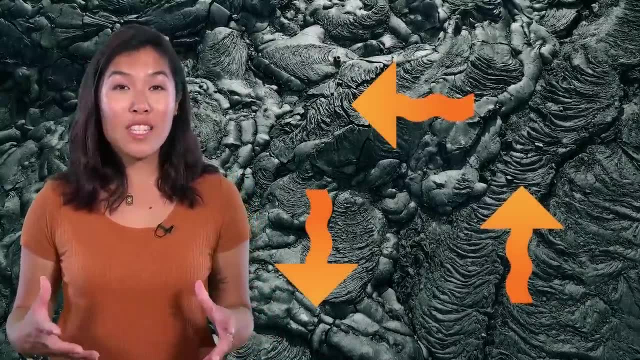 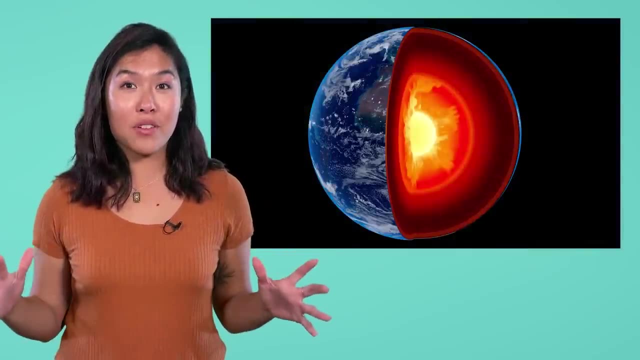 Although these rocks are in the solid state of matter, they actually flow like a very thick, slow moving liquid. This movement is caused by the currents of eukaryotes, which is the 열 intense heat in the mantle. The outermost edges of the mantle are over one thousand degrees Fahrenheit and the deeper 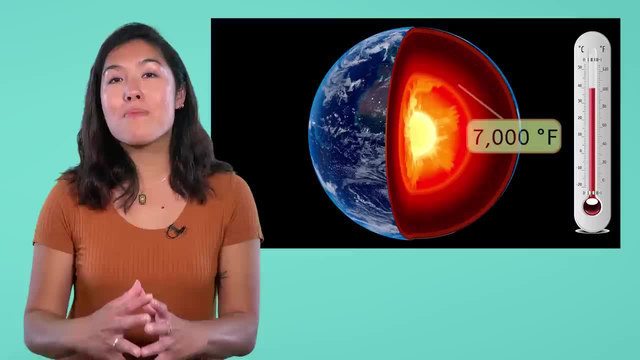 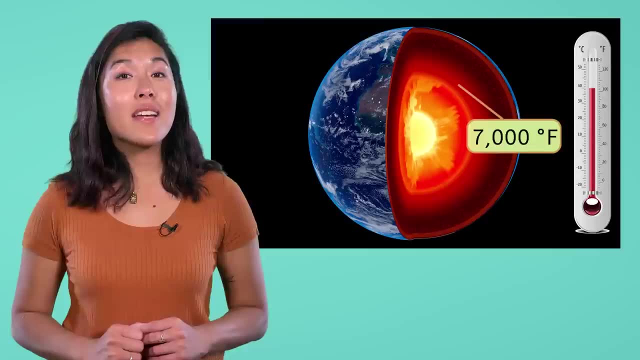 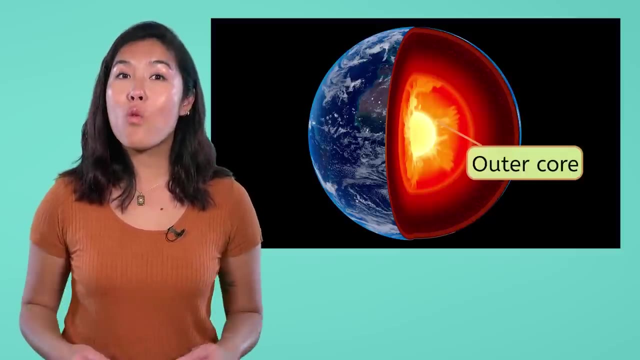 you go, the hotter it gets. The innermost parts of the mantle are over seven thousand degrees, But that's not nearly as hot as our next layer, the outer core. The outer core is about one thousand four hundred miles thick and it's mostly made. 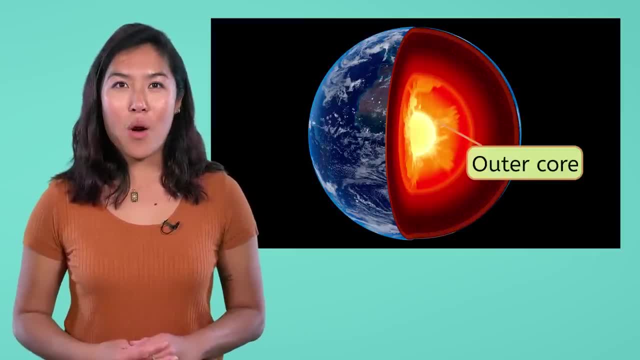 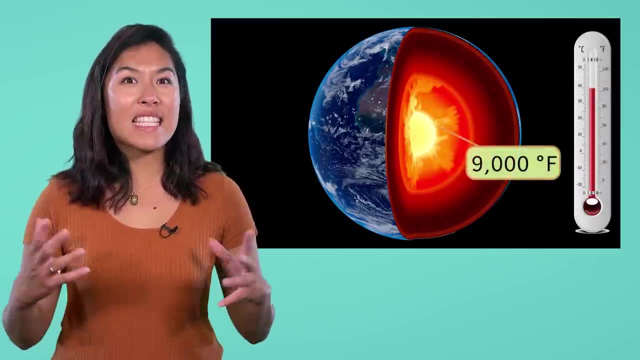 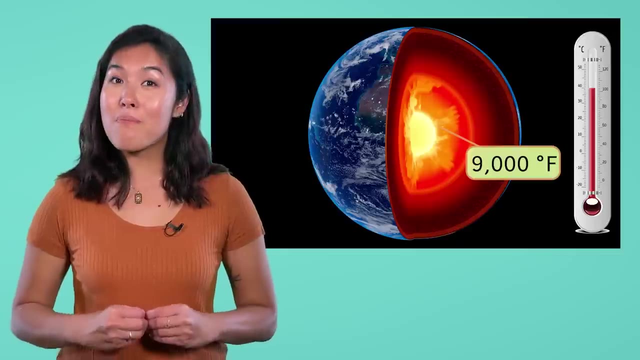 of the metals iron and nickel. Now remember: the deeper into the Earth we go, the hotter it gets. The outer core reaches temperatures as high as nine thousand degrees Fahrenheit. So how do you think these high temperatures impact the metals that make up the outer core? 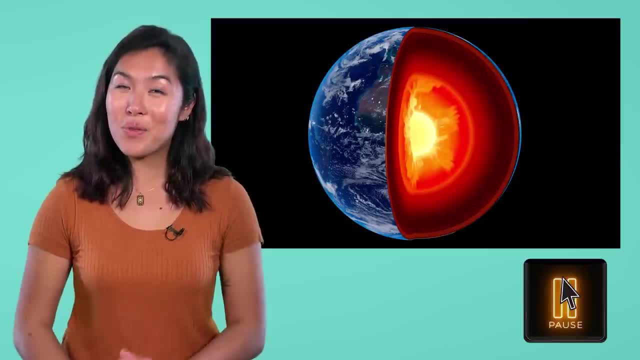 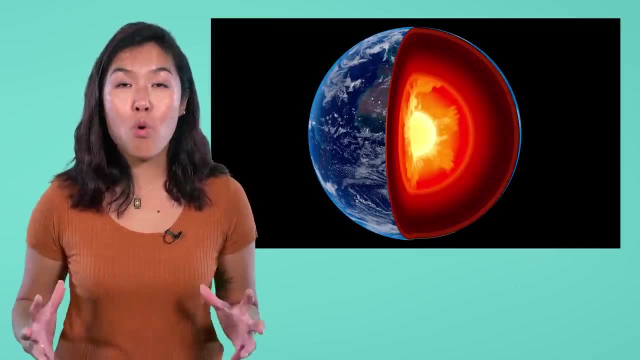 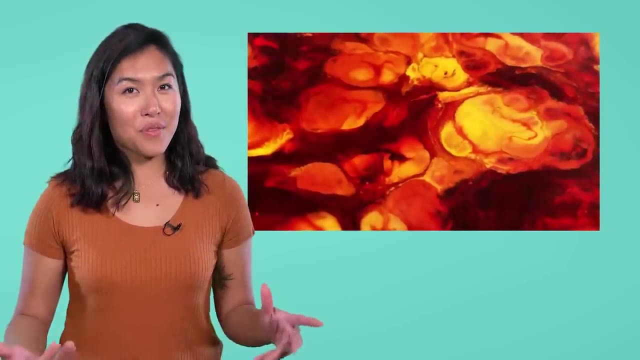 Pause the video here and record your thoughts in your guidebook. The scorching temperatures of the outer core are well past the melting points of the metals found here. As a result, the outer core isn't solid rock like the mantle and crust. 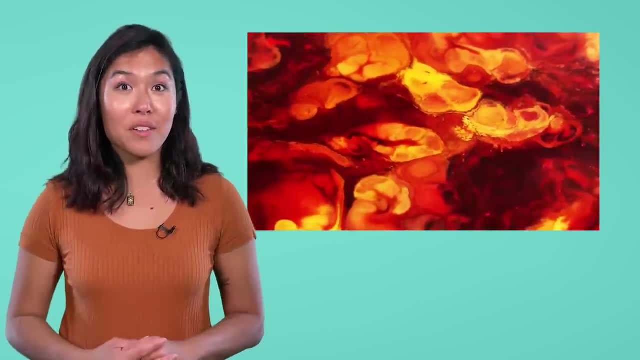 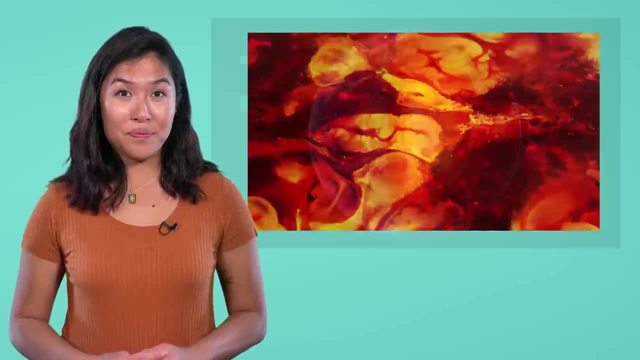 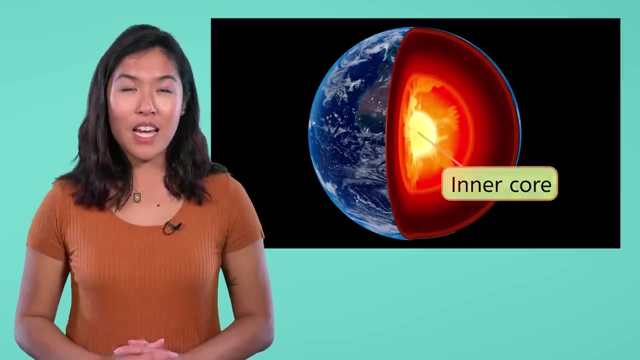 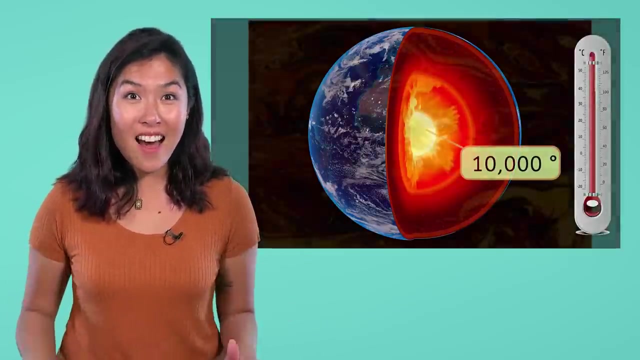 Instead, it's made of molten liquid metal And there's one last layer that's even deeper: The inner core. The inner core is a dense ball of iron about seven hundred fifty miles across. It's close to ten thousand degrees Fahrenheit, making it as hot as the surface of the sun. 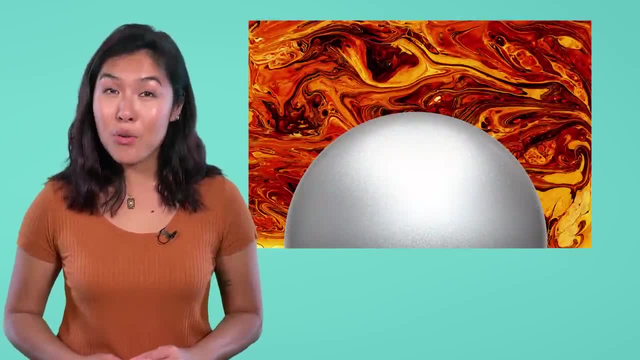 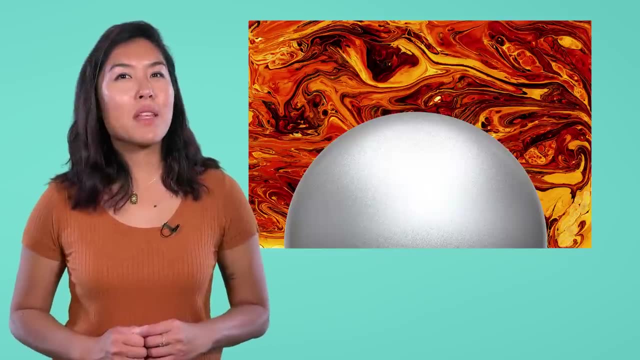 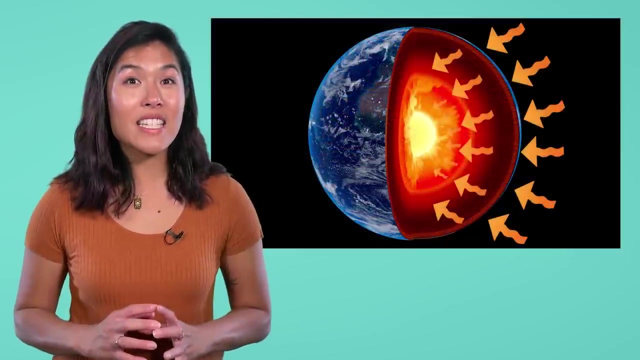 But despite being even hotter than the molten outer core, the inner core isn't liquid, It's completely solid. What do you think is keeping the metal here from melting The inner core? The inner core is solid. Remember, the inner core has an entire planet pressing in on it. 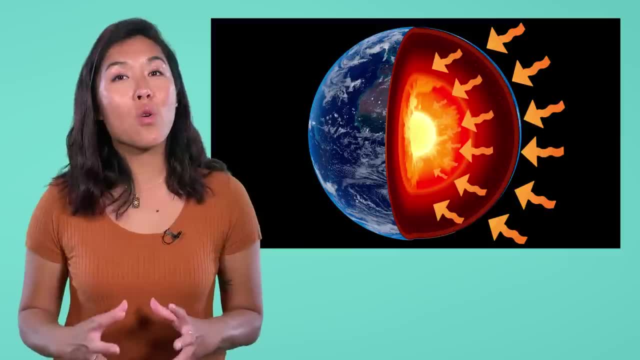 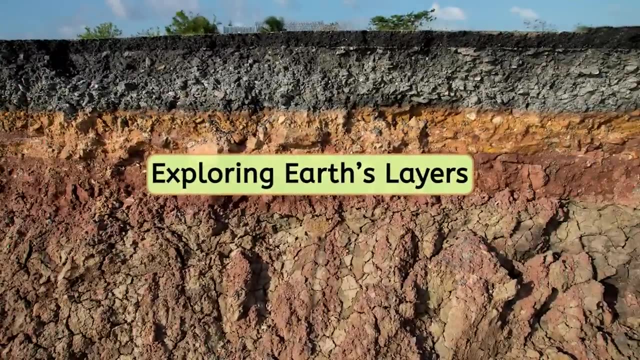 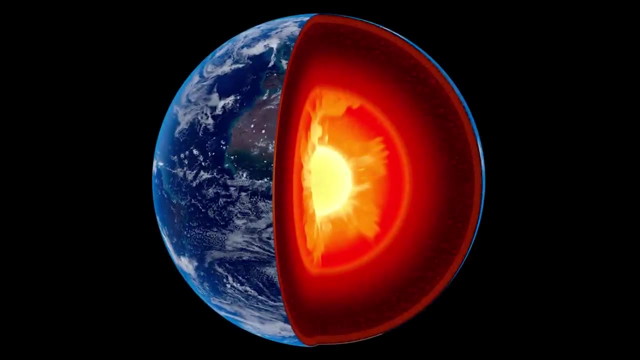 Even though it's definitely hot enough to melt iron, the inner core stays solid because of the incredible amount of pressure it's under. Our best efforts to explore Earth's layers have barely scratched the surface of our planet. We've made a lot of progress. 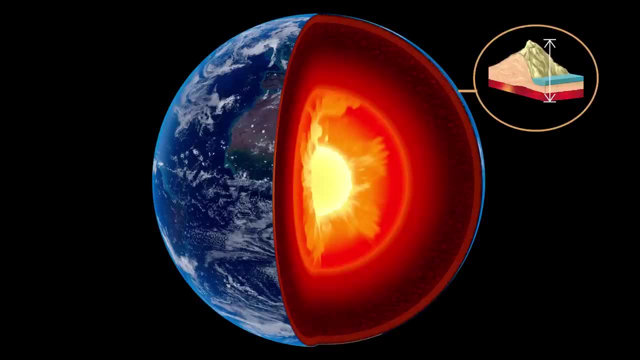 We've made a lot of progress. We've made a lot of progress. We've made it less than halfway through the crust, and it doesn't look like we'll be getting much deeper any time soon. So what do you think it is that makes exploring the planet's inner layers so challenging? 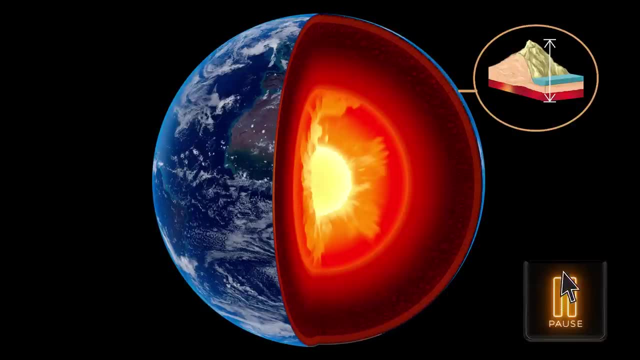 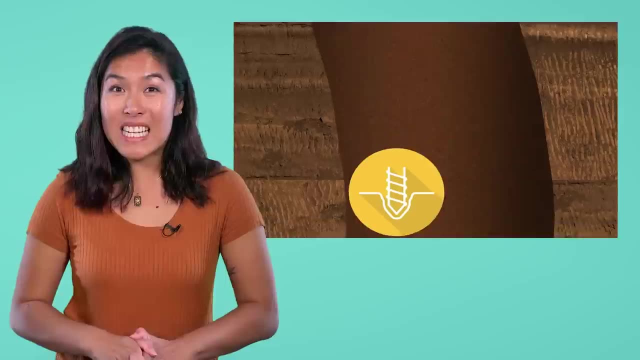 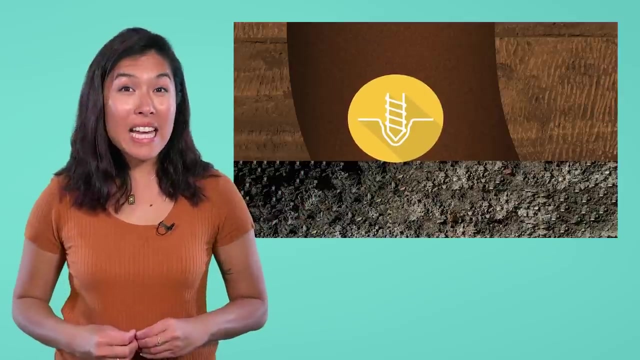 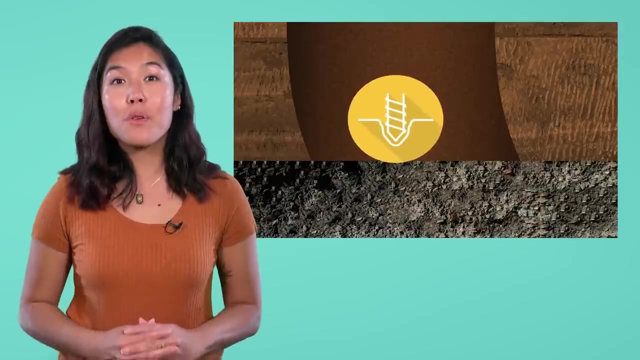 Pause the video here and record your thoughts in your guided notes. Firstly, reaching our planet's inner layers entails drilling through several thousand miles of solid rock. But even if we can get through the rock, there's the problem of the high temperatures. In fact, this is why the Kola Superdeep Borehole stopped at around 40,000 feet down.